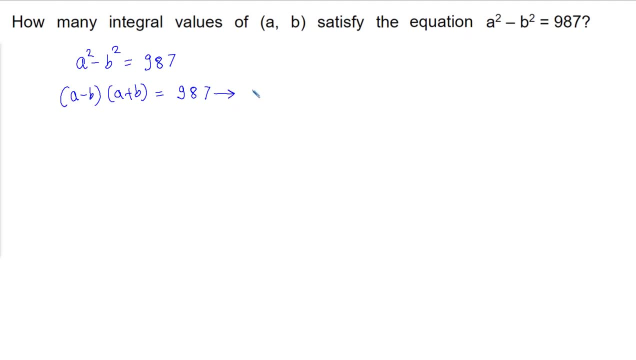 so, let's do the prime factorization. Let's do the prime factorization. This is nothing but what? 3 into 3 into 327.. Okay, 3 into sorry, 3 into 329.. Okay, so now 327 is equal to 987.. Okay, so, let's do the prime factorization. Let's do the prime factorization. 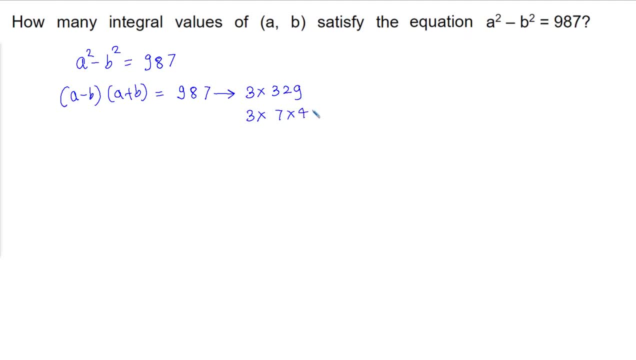 329 is 7 into 7 into 47.. Okay so the prime factorization is 3 to the power 1 into 7 to the power 1 into 47 to the power 1.. Okay so, how many factors this number is having the number of? 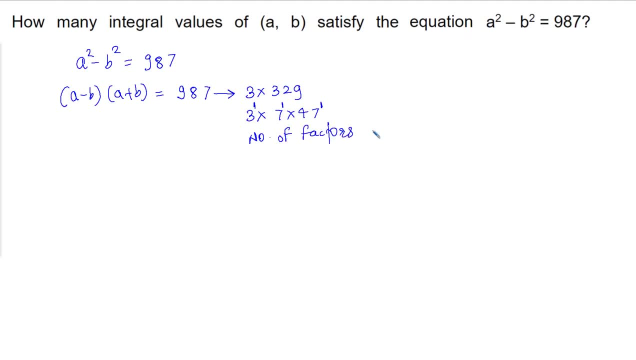 factors. the number of factors are 1 plus 1 into 1 plus 1 into 1 plus 1.. Okay, that is equal to how much 2 into 2 into 2.. Okay, that is equal to how much total number of factors are 8.. Okay, everyone. 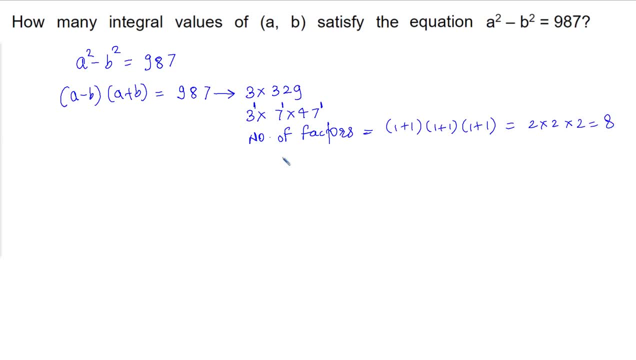 2 into 2 into 2, that is equal to 8.. so now, in how many ways? in how many ways we can express 987 as a product of two numbers, first number and second number? in how many ways we can express 987 as a product of two numbers, that is? 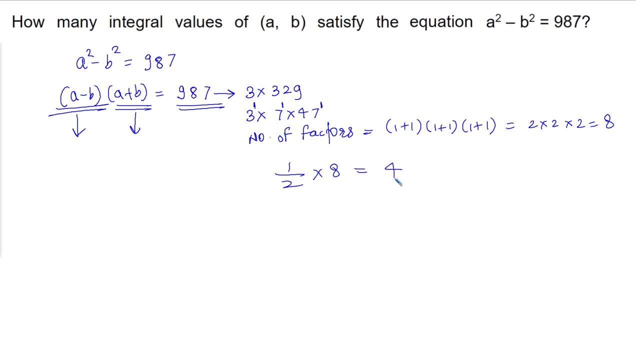 half into eight. okay, half into eight is how much four? there are four ways in which we can express 480: 987. okay, there are four ways in which we can express 987 as a product of two numbers. okay, everyone now, for example, for example, you can see that. you can see that out of these four ways, 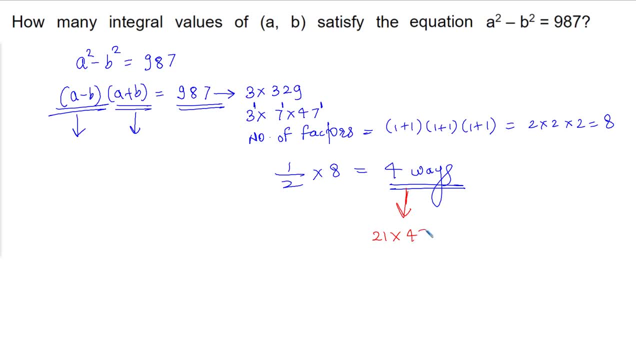 one of the ways 21 into 47: okay, everyone now. one of the ways 21 into 47: okay, everyone now. so this 21 into 47. we can write it as 47 into 21. okay, we can also write it as minus 21 into minus 47. 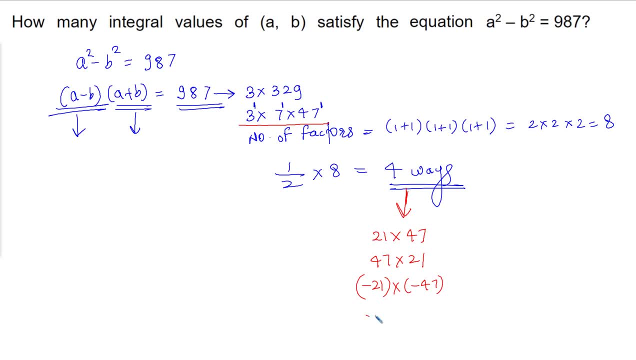 okay, everyone. and we can also write it as minus 47 into minus 21. okay, everyone. so now, first number means the value of a minus b and the second number means the value of a plus b. so the one way will generate four different possible solutions. okay, everyone. so, total: there are four ways, are there? 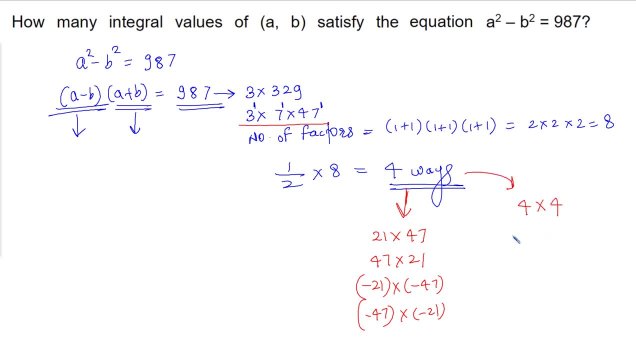 okay, and every way will generate four different combination. so total number of solutions are going to be how much? total number of solutions are going to be 16, okay, everyone. so the answer is going to be 16, because we need to consider the reverse also and we need to consider: 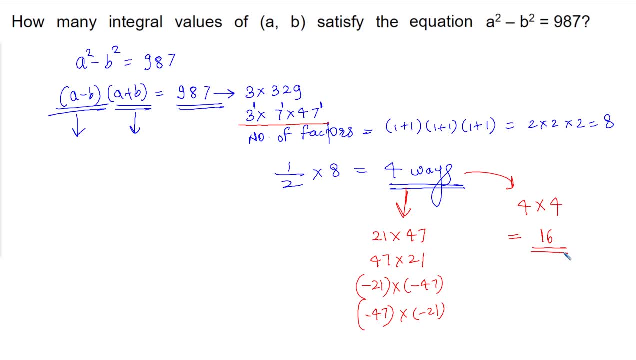 negative also, because over here, we are not interested only in positive integral solutions, okay, we are interested in negative integral solutions also, okay, that is why we need to take the reverse possibility also and we need to consider the negative possibilities also, okay. so over here, the final answer is 16. let's do one more question. okay, how many integral values x? 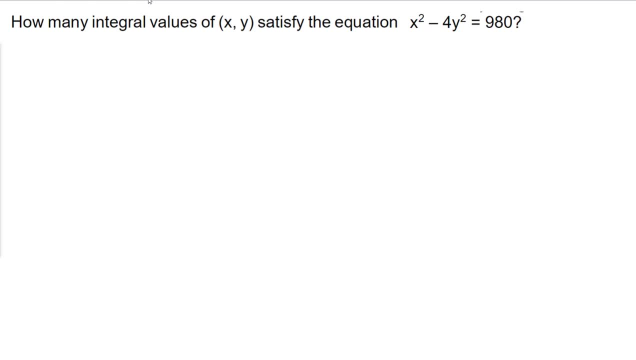 comma y. okay, how many integral values of x comma y satisfy the equation? equation: x square minus 4y square is equal to 980. okay, everyone. so let's do the factorization over here. the factorization is what x minus 2y into x plus 2y. this is equal to how much? 980 okay. 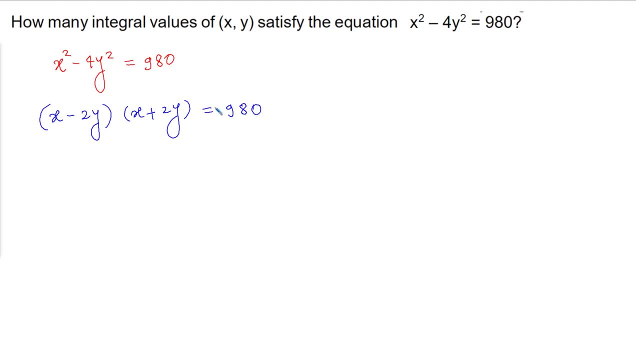 the product of these two bracket is 980. that is equal to product of these two brackets. is even number. okay, means at least one of the two bracket has to be one number. okay, if i consider first bracket as even second bracket automatically becomes even, as we did in previous question. okay, 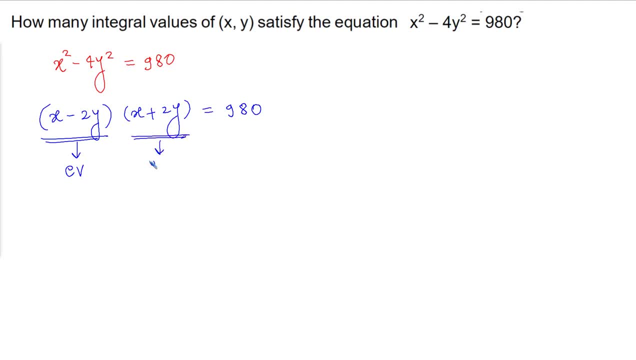 so if first bracket is even, second bracket is automatically even, or second bracket is even, then first bracket is automatically even. okay, so first the both brackets are supposed to be even number. okay, so even into even is how much 980? okay, every even number is in which format? 2 into. 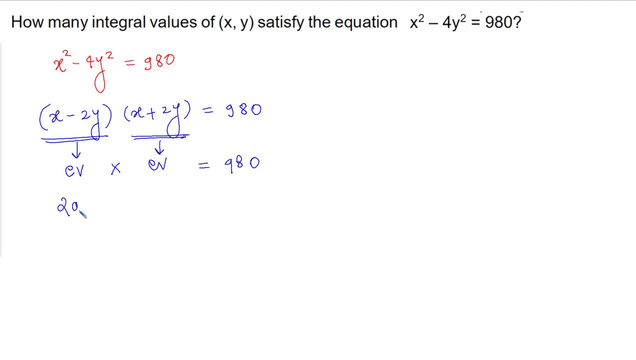 something. so first bracket, let's consider it as 2 into a, and the second bracket, let's consider it as 2 into b. okay, so 2 into a into 2 into b is equal to 980. okay, so let's consider it as 2 into. 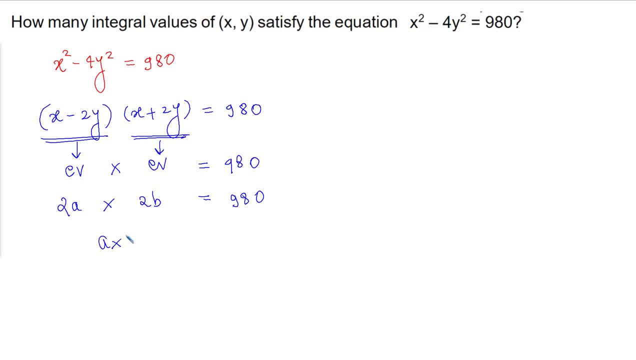 to how much 980. so value of a into b becomes how much? okay. 980 divided by 4. so the value of a into b becomes how much? 4, 2, 8, 4, 4, 16 and 4, 5, 20, okay, so the value of a into b is equal to how much? 245? 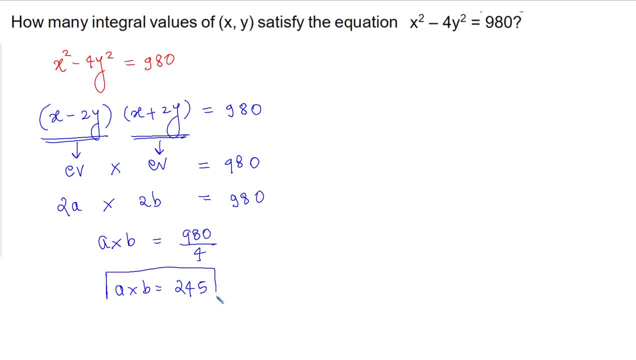 now, how many integral solutions are there for a into b is equal to 245. okay, let's find out that. let's do the prime factorization of 245. 245 is equal to how much? 5 into 5 into 49? okay, that is equal to 5 into 7 square. let's find the number of factors. okay, the number of factors is equal.